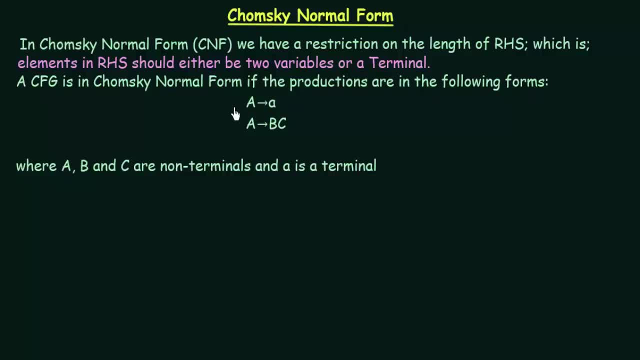 Okay, so let's see here All the productions are in the following forms: So here we have two productions given, and let's see the first one. The first one says A gives small a. Here this capital A is a variable or a non-terminal symbol, and this small a is a terminal symbol. 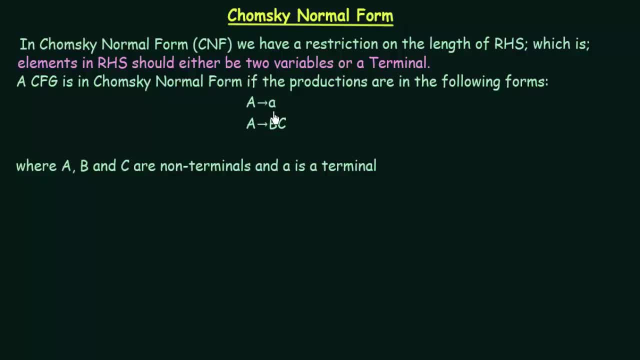 So we see that in the RHS there is just a single a, which is a terminal symbol. So if there is a single terminal symbol then it is in Chomsky Normal Form, And in the second production here it says A gives BC. 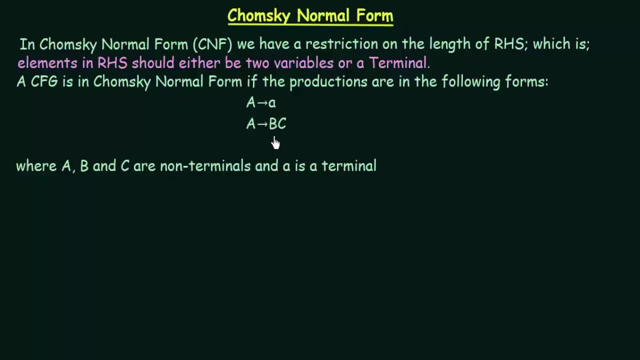 Here both B and C are variables or non-terminal symbols. So in the RHS if we have two variables, then also it is in Chomsky Normal Form. So all productions which are in this form are said to be in a Chomsky Normal Form. 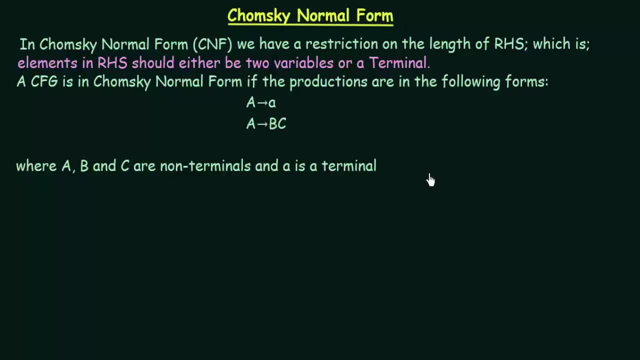 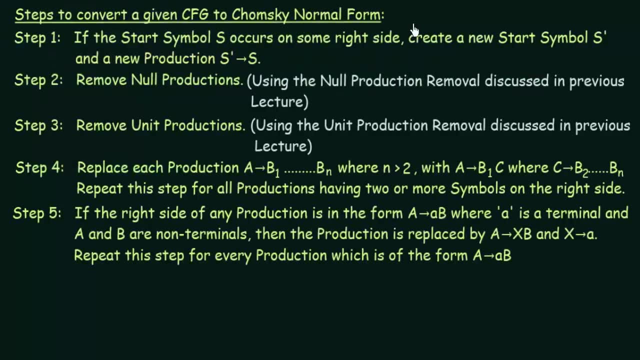 Alright, so now we will see the steps that we need to follow in order to convert a given CFG to its equivalent Chomsky Normal Form. So here are the steps. We have steps 1. 1-5, and following these five steps, we can convert a given CFG to Chomsky normal form. 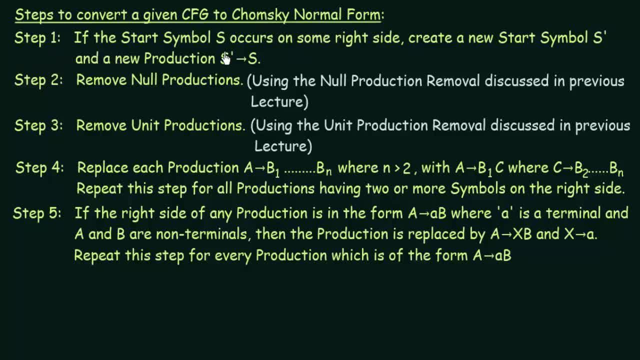 So let's see the steps. Step number one: If the start symbol s occurs on some right side, create a new start symbol s- turf and a new production s- gives s. So if the start symbol occurs on the right side of some production, then we have to create a new start symbol s- turf. 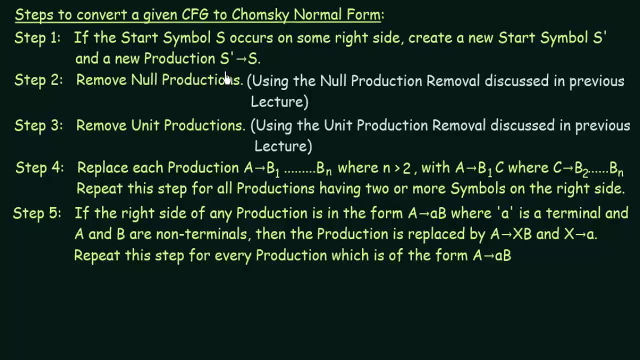 And also we will create this new production for that. saying S dash gives S, So you have to perform this- step number one if you are having a start symbol on the right hand side of any of the productions. Step two: remove null productions. So in the last lecture I have taught you how to remove null productions. So following 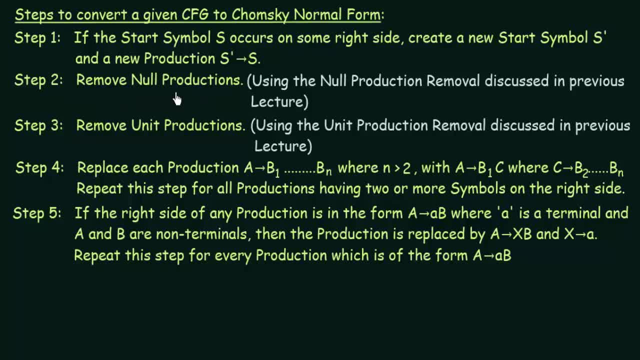 those steps. you have to remove the null productions, if there are any, using the null production removal discussed in the previous lecture. And in step three, you have to remove the unit productions. This also I have discussed in the previous lecture. So, using the unit production removal discussed in the previous lecture, you have to remove all the unit productions. 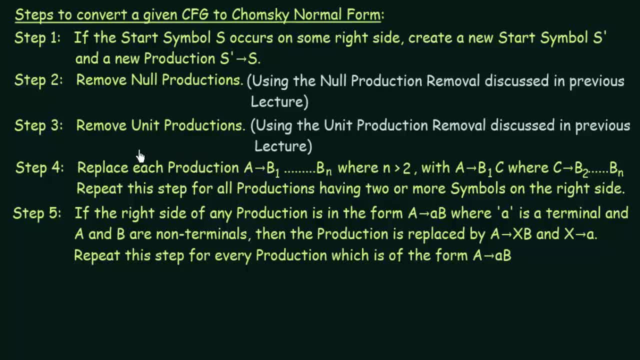 in the CFG, if there are any, All right. so, coming to step four, it says: replace each production: A gives B1, B2 up till Bn, where n greater than 2, with A gives B1, C where C gives B2 up till Bn. Repeat this step for all productions having. 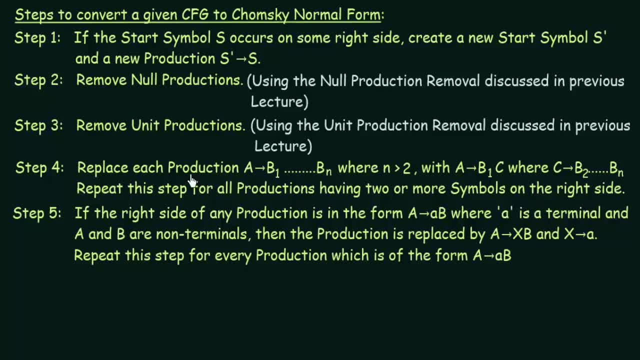 two or more symbols on the right side. So we already saw that in the definition of Chomsky normal form in the right hand side we are allowed to have only two variables. So if you are having a production of this form where on the right hand side you are having n variables, 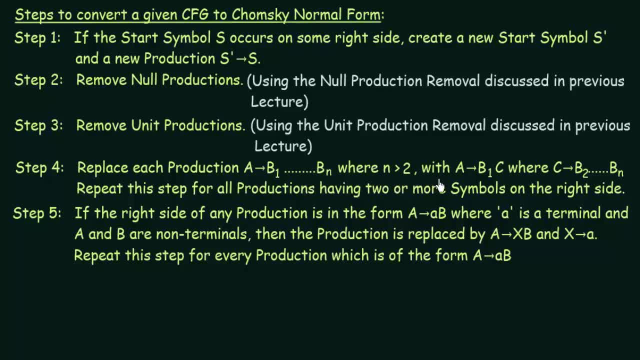 So here n is greater than 2.. So what you have to do, you have to create productions of this form: A gives B1, C, so that in the right hand side we will have only two variables and here C will give B2. that means, here we have taken B1, remaining one was B2 till Bn, So C will. 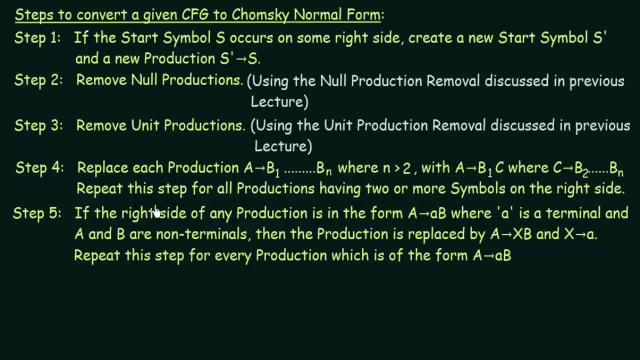 give B2 till Bn. So you have to repeat this step for all productions having two or more symbols on the right side. So as you repeat this, you will reach a stage when you will have only two variables on the right side of each production. So till you reach that stage, you have to do this step. 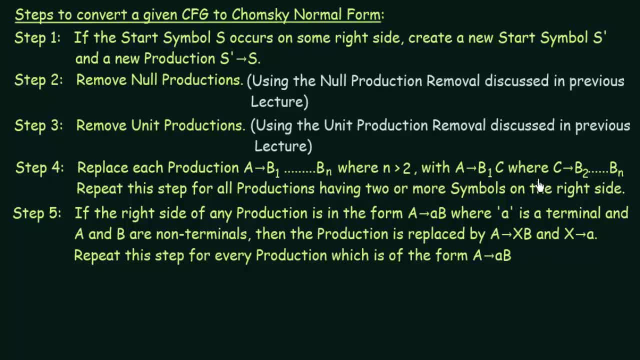 number four. Ok, so don't worry, even if this seems a little confusing, it will be clear when we take example in the next lecture. Ok, so after performing step four, we come to step five, in which it says: if the right side of any production is in the form A gives AB. 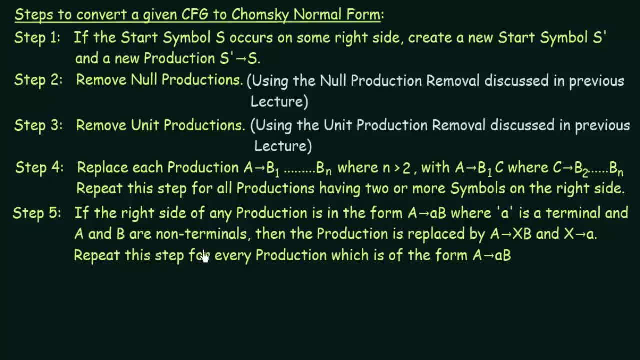 where A gives AB. So if the right side of any production is in the form A gives AB, where A is a terminal and A and B are non-terminals, then the production is replaced by A gives XB and X gives A. Repeat this step for every production which is of the form A gives AB. 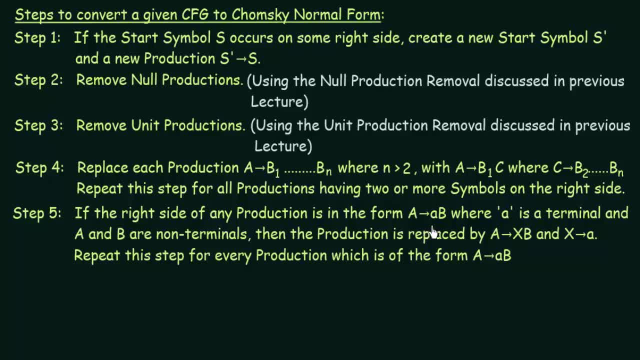 So we saw in the rules of Chomsky normal form that we can have either one terminal symbol in the right hand side or two non-terminal symbols. but symbols of this form, where there is one terminal symbol and one non-terminal symbol, are not in the form. So we have to.